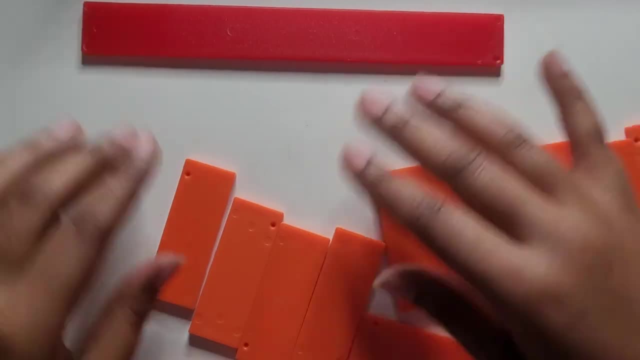 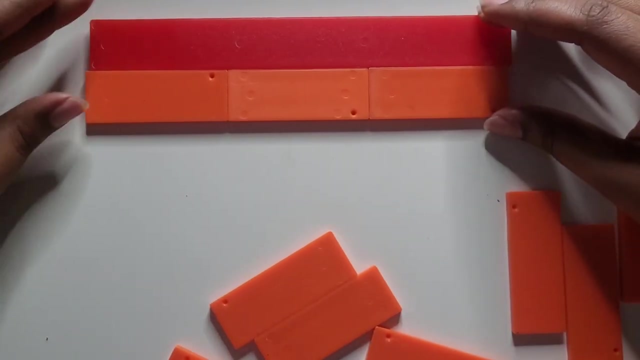 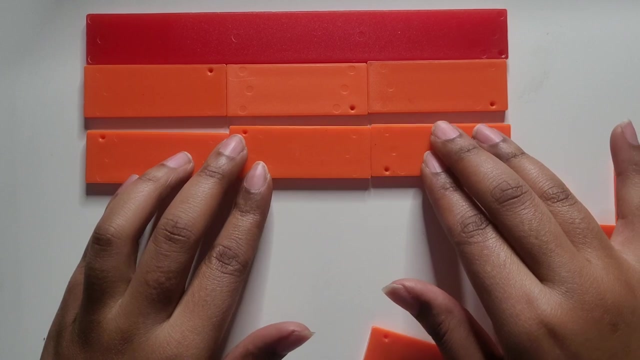 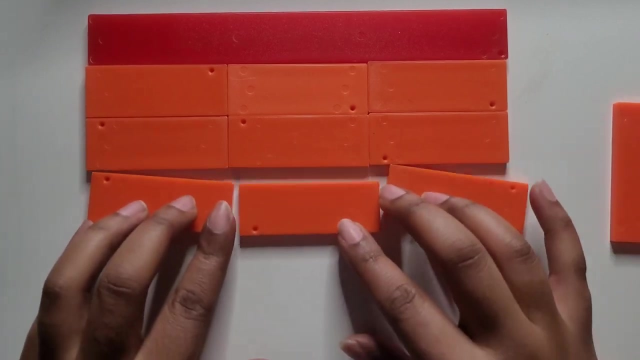 into a mixed number. So let's think about how many thirds is equivalent to one whole. Lining up our thirds against the red tile, which represents one whole, we see that three thirds is equivalent or equal to one whole. Let's continue to do. 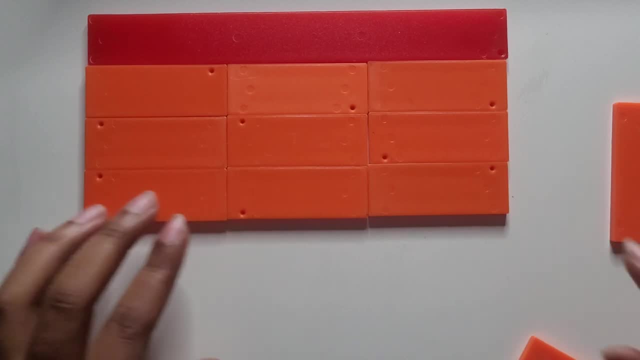 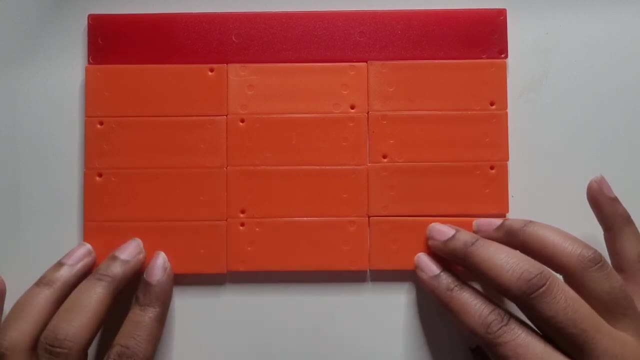 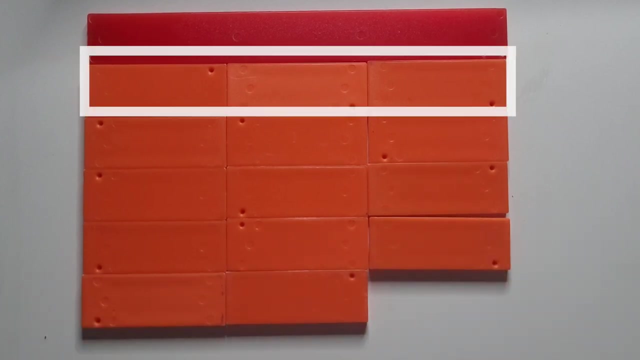 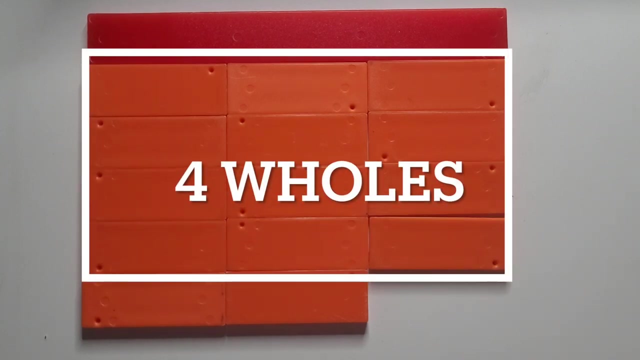 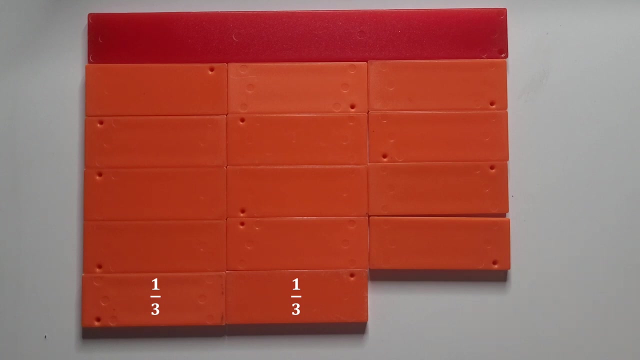 that until we use all of the 14 thirds. Now that all of the thirds are grouped into wholes, let's count how many holes we made: One, two, three, four. We made four wholes from the fourteen thirds. And remember they're an extra two thirds. We don't have enough to make. 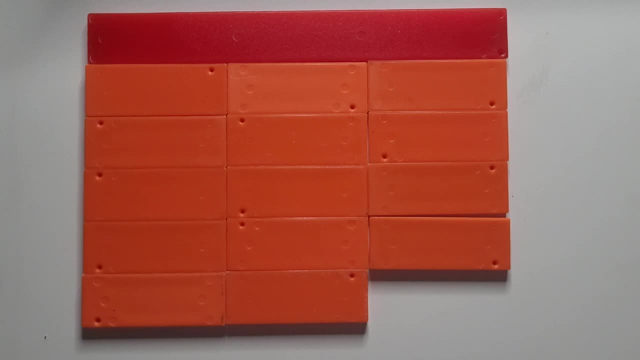 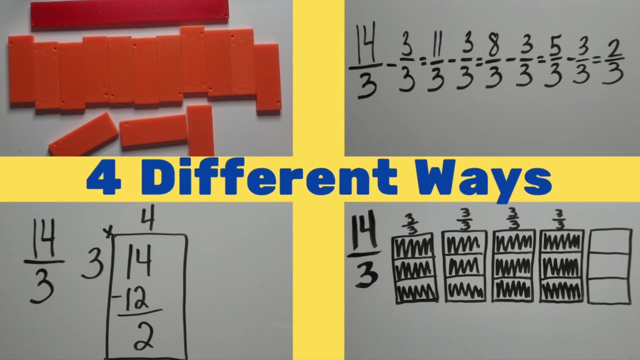 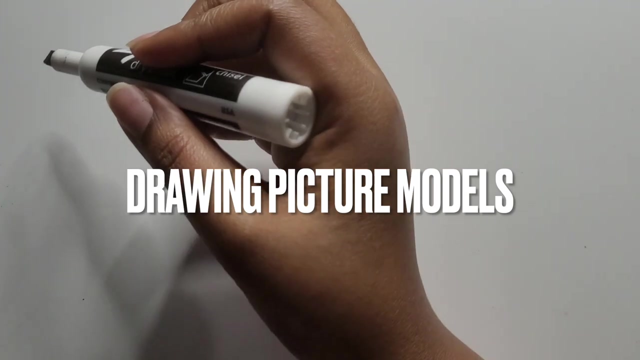 another whole. So what is our new mixed number Four and two thirds? Fourteen thirds is equal to four into thirds. The second way we will look at converting a fraction greater than 1 into a mixed number is by drawing picture models. We're going to use the 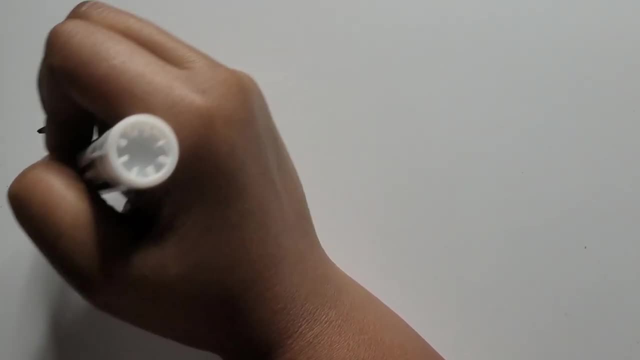 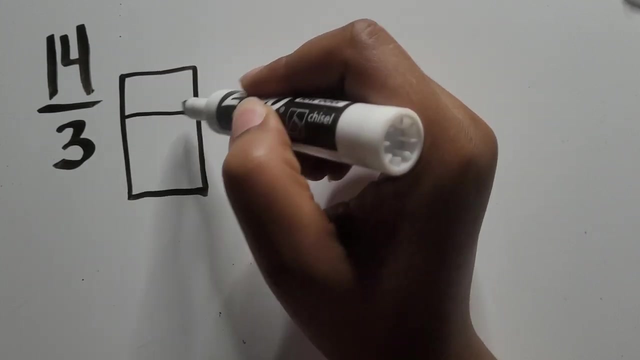 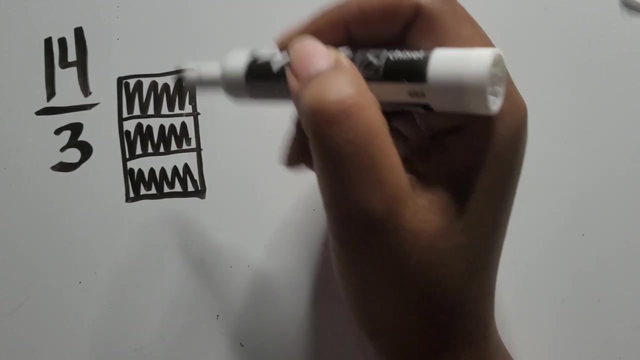 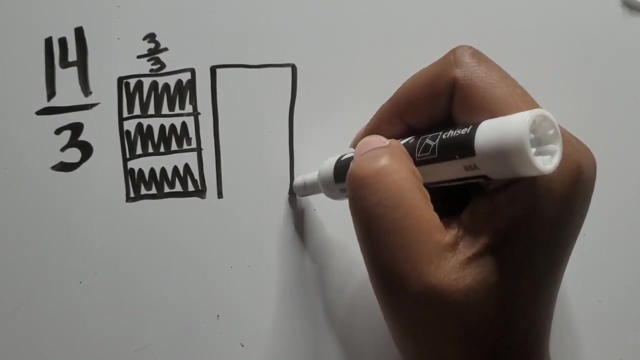 same fraction, 14 thirds in this example, Similar to using the fraction tiles, we'll need to think about how many thirds is equal to one whole and represent that in the picture model we draw. Again, we see that three thirds makes up one whole. Let's repeat what we. 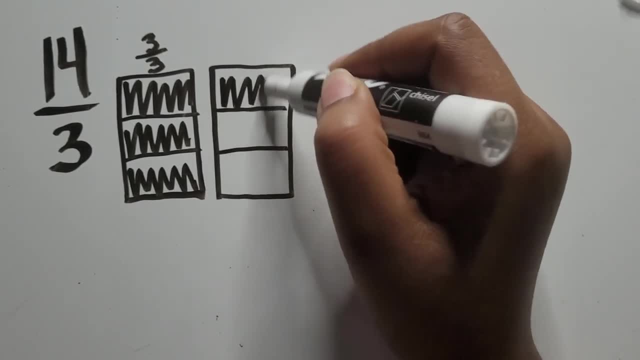 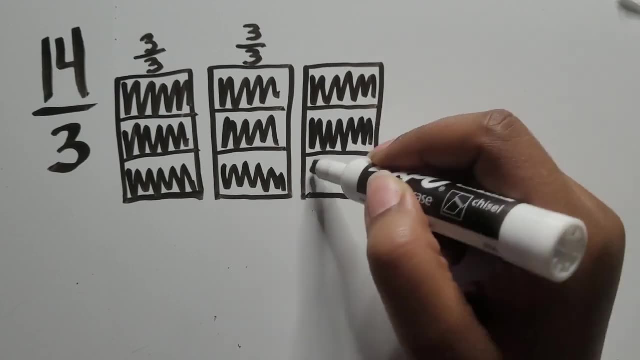 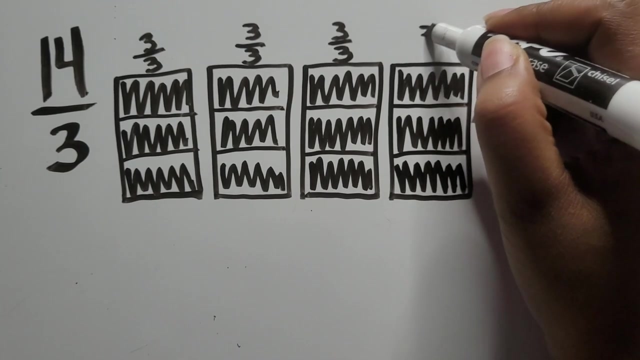 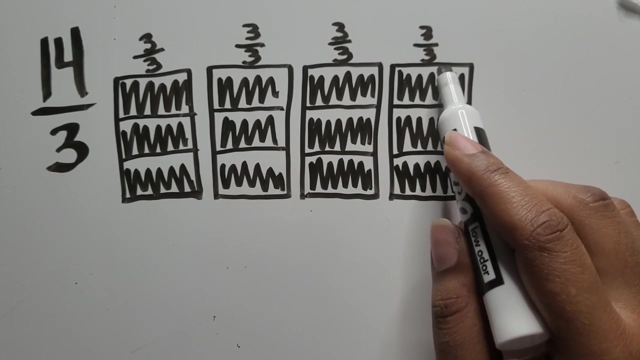 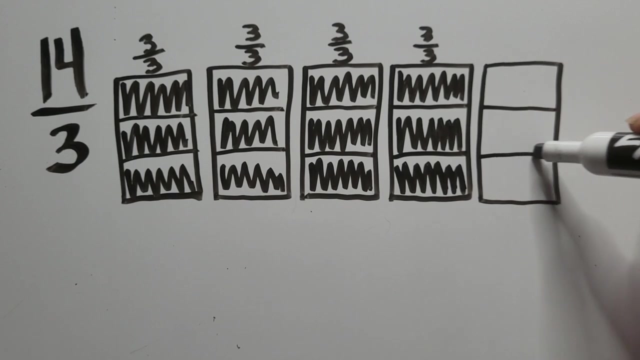 just did to show a total of 14 thirds. So far we have four groups of three thirds: Three thirds and three more is six thirds, three more is nine thirds and three more is twelve thirds. We'll have to draw an extra whole to get to 14 total thirds, But we'll only shade in two. 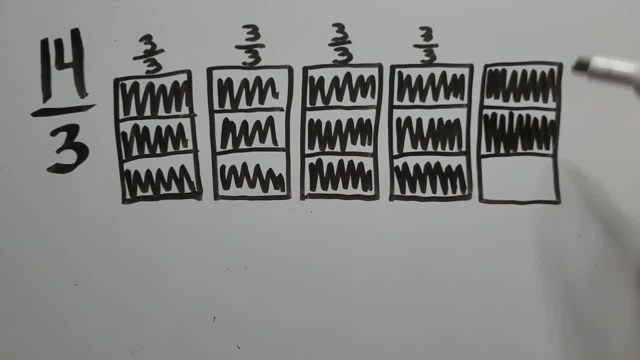 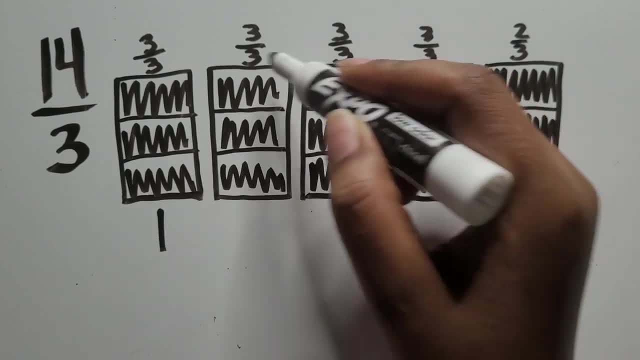 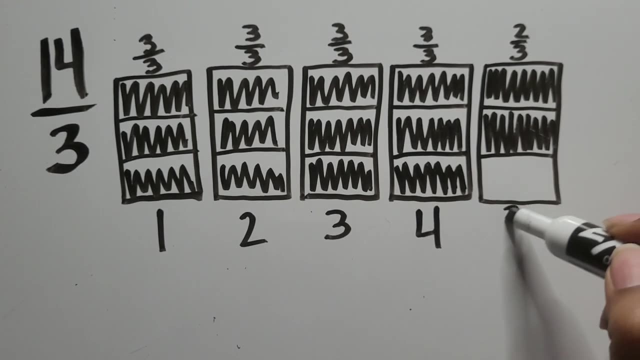 of the thirds, because we don't need all three to get to 14 thirds. Now let's count how many holes that are equal to one whole. We'll start completely shaded in one, two, three, four holes and two extra thirds are. 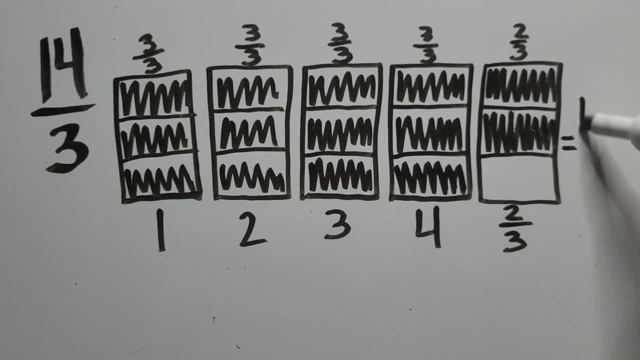 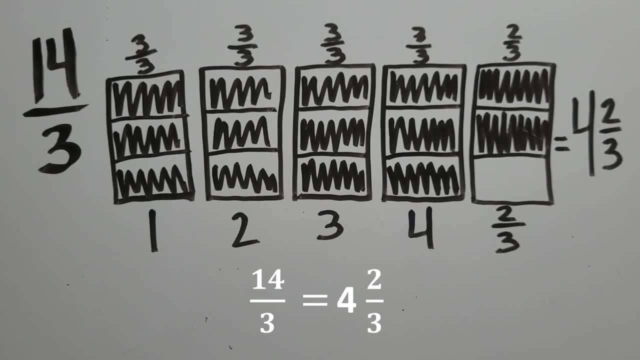 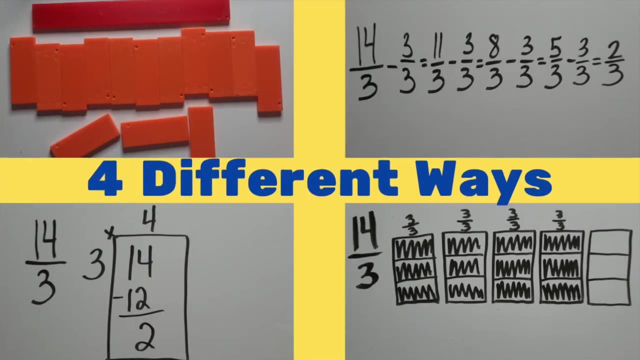 shaded in. So with this model, we see that we have a total of four holes and two thirds. Fourteen thirds is equal to four and two thirds. Our third way moves away from pictures and focuses on using repeated subtractions. We'll use the fraction as a way to convert a fraction greater than one to a. 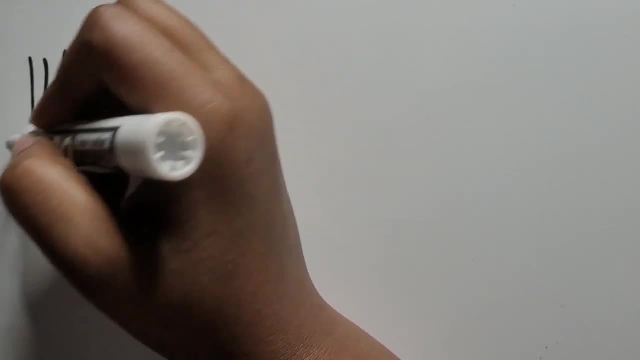 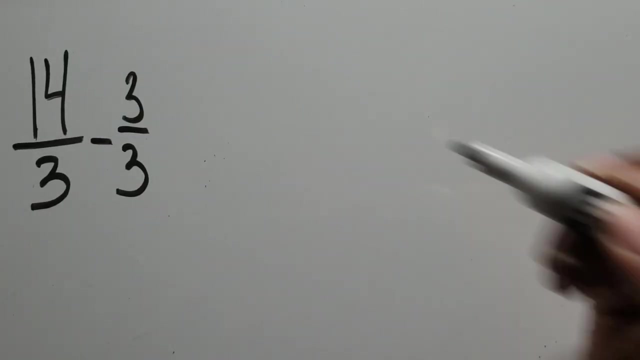 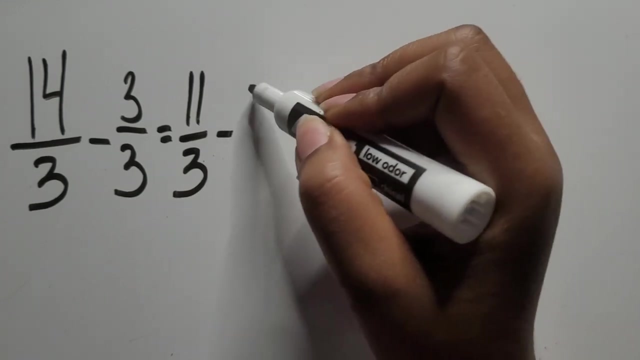 mixed number. Again, we're using the example of 14 thirds to highlight these strategies. With repeated subtraction, we want to subtract out a whole or the amount of thirds that equals to one whole, and that is three thirds. Fourteen thirds minus three thirds is eleven thirds. Eleven thirds minus three thirds. 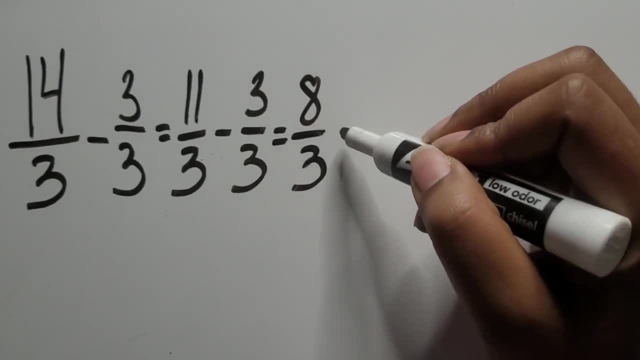 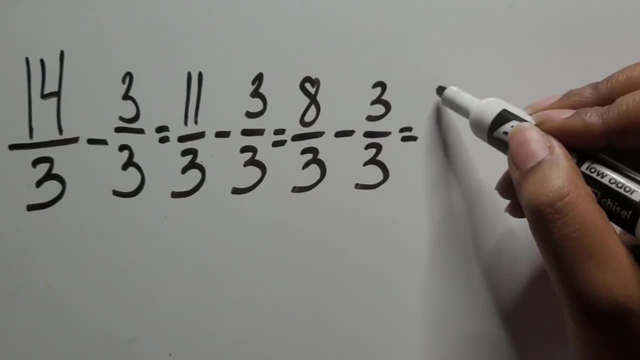 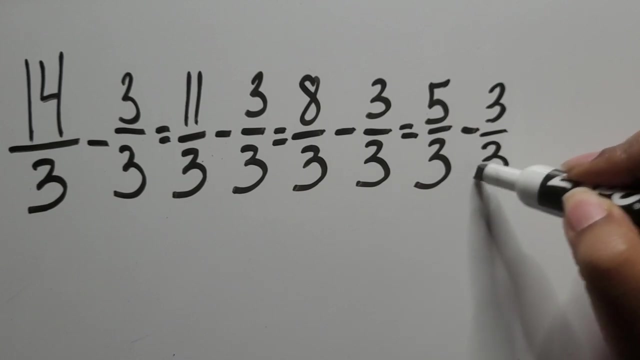 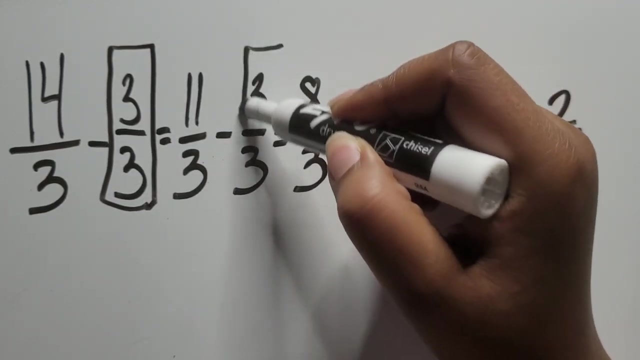 is eight thirds. We can continue doing this until we no longer can subtract three thirds. Remember that is how much is equivalent to one whole. in this example, With two thirds being left over, it's not enough to subtract another three thirds, so we'll stop here To count how many holes are in fourteen thirds. let's group: 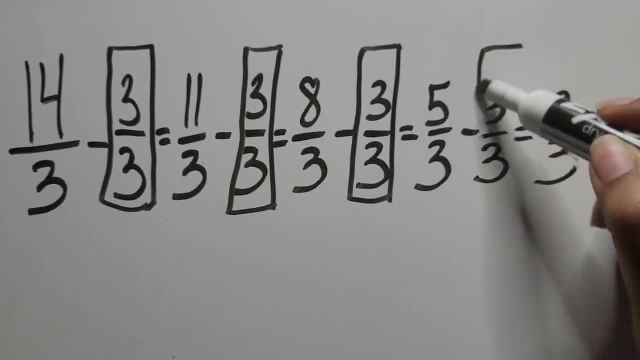 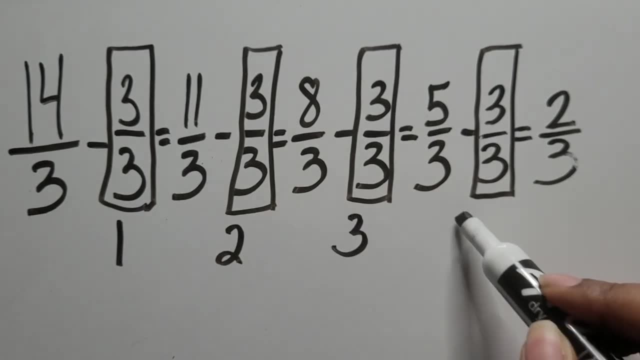 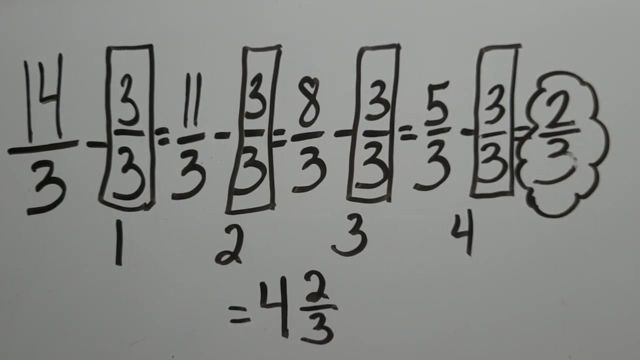 each three thirds that we subtracted and see how many there are in total: One, two, three, four. There are four holes in fourteen thirds and two extra thirds. Don't forget those extra thirds. Fourteen thirds is equal to four and two thirds. 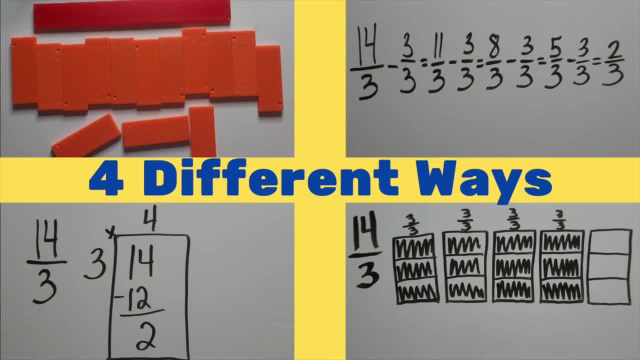 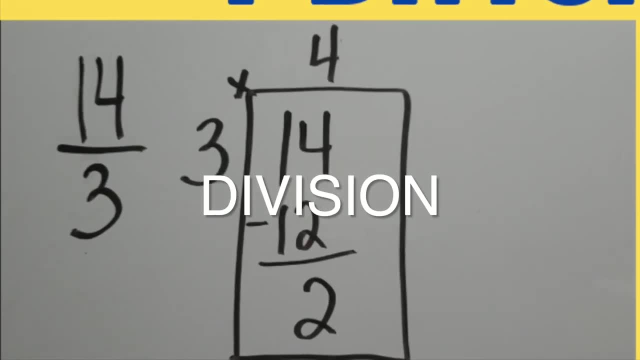 In the fourth way of showing how to convert fractions to numbers, we'll use the same method. Knowing how to convert fractions greater than one to a mixed number, we'll use division. When using division, choose the division strategy that you or your students are most comfortable with. 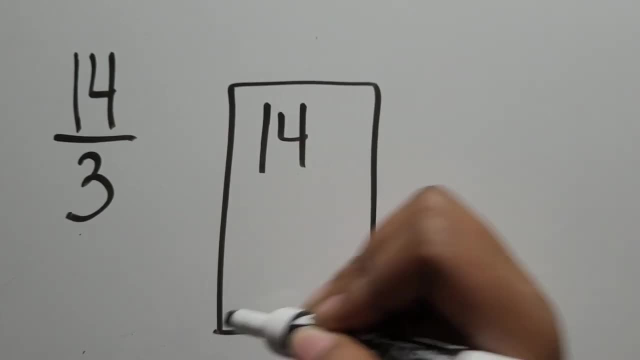 In this example we're using partial quotient, which can look very similar to long division. just ensure that students understand that we're dividing 14 by 3, or the numerator by the denominator. When dividing 14 by 3, we can think about there being four groups of 3 and 14, and four times three equals four thirds and two fifths of a third. Then we can use divisional division to dollar the number of fractions we've divided by the denominator. When dividing Ti by 3, we can think about there being four groups of three and fourteen and four thirds on one inom.